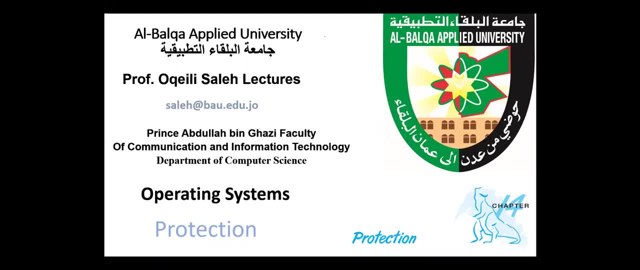 Hello everyone. Today we start Unit 5 in Operating Systems course, and this unit consists of two chapters: Protection and Security. Protection refers to a mechanism for controlling the access of programs, processes or users to the resources defined by a computer system. 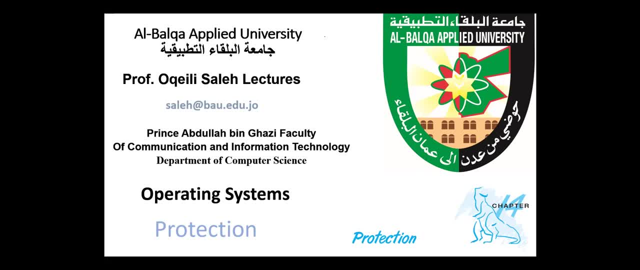 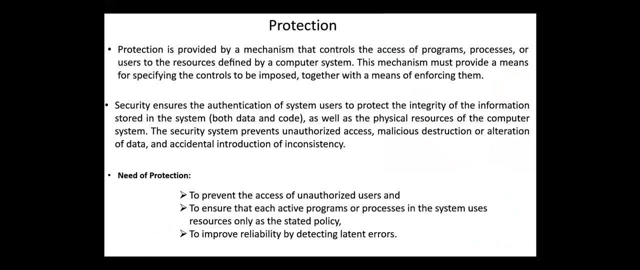 While security is a measure of confidence that the integrity of a system and its data will be preserved, Today we start with protection: the need for protection, its goals and the principles of protection. Protection is provided by a mechanism that controls the access of programs, processes or users to the resources defined by a computer system. 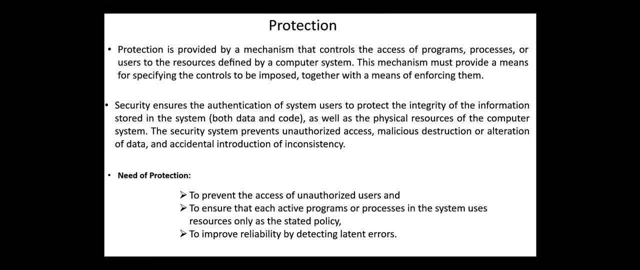 Protection is provided by a mechanism that controls the access of programs, processes or users to the resources defined by a computer system. This mechanism must provide a means for specifying the controls to be imposed, together with a means of enforcing them. Security ensures the authentication of system users to protect the integrity of the information in the system, both data and code, as well as the physical resources of the computer system. 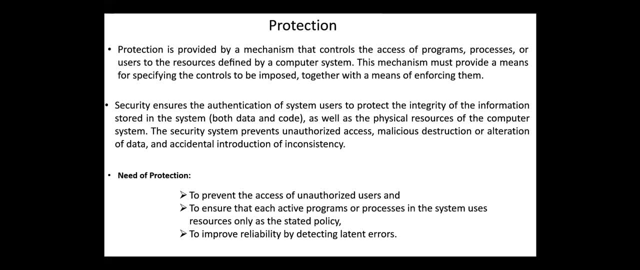 The security system prevents unauthorized access, malicious destruction or alternation of data and accidental introduction of inconsistency from the Chinese. IoT Protection shall prevent the access of unauthorized users and ensure that each active program and process in the system is only plied with resources. the policy stated 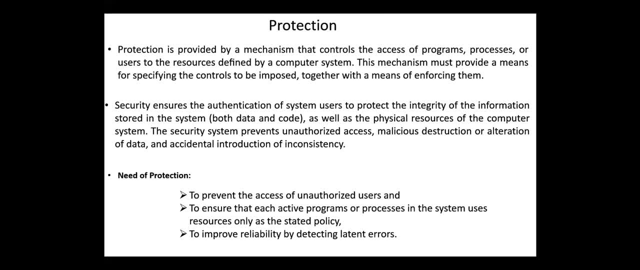 It will not improve reliability while detecting latent errors. The goals of protection are: to protect maliciousabộrtoions from Homeland Security and er convexities against those that govern the system. To prevent maliciousabộrtoions from Constellations and Dolor rasions against those that govern the system. 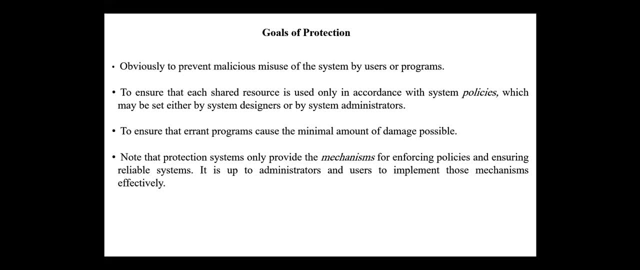 use of the system by users or programs. to ensure that each shared resource is used only in accordance with the system policies, which may be set either by the system designers or by the system administrators. to ensure that errant programs cause the minimal amount of damage possible.